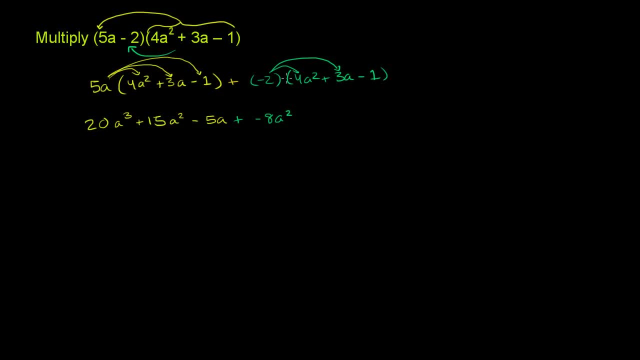 So we just did that: Negative 2 times 3a, Negative 2 times 3 is negative 6a. And then finally you have negative 3a, Negative 2 times negative, 1.. Well, negative times, the negative is a positive. 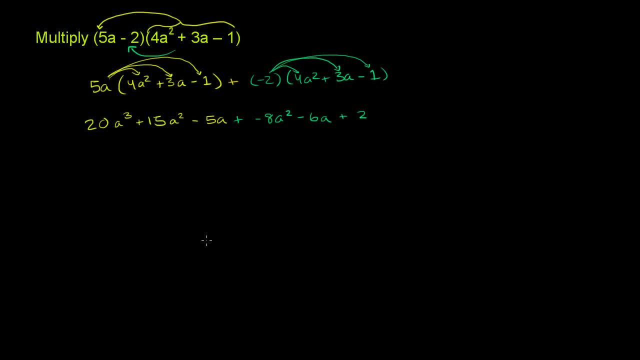 So that is positive 2.. And now we can combine like terms. We only have one third degree term over here. We only have the 20a to the third, So let's just write that down: 20a to the third. 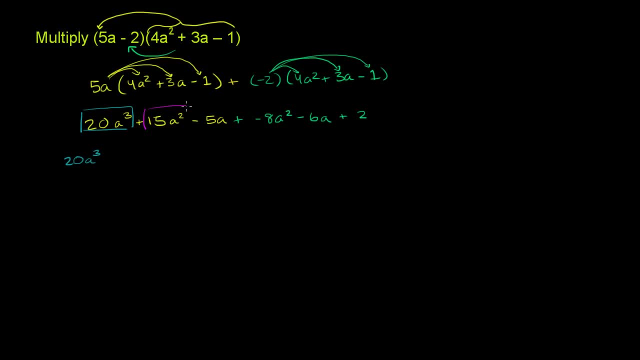 And then let's look at our a squared terms. We have a 15a squared term right over here And we have another negative 8a squared. So if I have 15 of something and I subtract 8, if I subtract 8a squared, I get negative 8a squared. 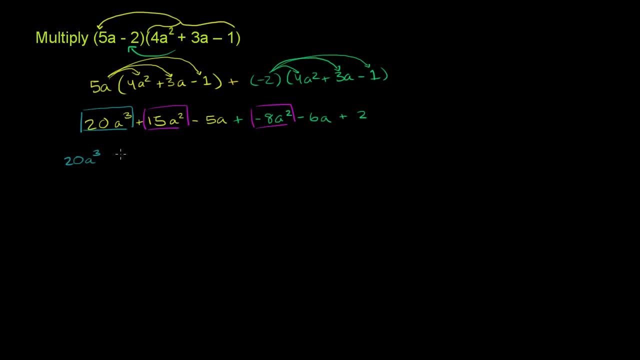 If I subtract 8 from that, then I have 7 of that something left. So 15 minus 8 is 7a squared, And then we have- let me do a new color here- We have a negative 5a. 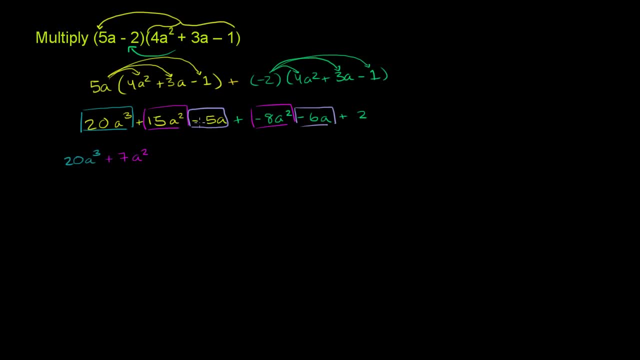 And to that we're going to add a negative 6a, So we're already negative 5.. We're going to get another negative 6.. We're going to become 6 more negative, So that is negative 11a. 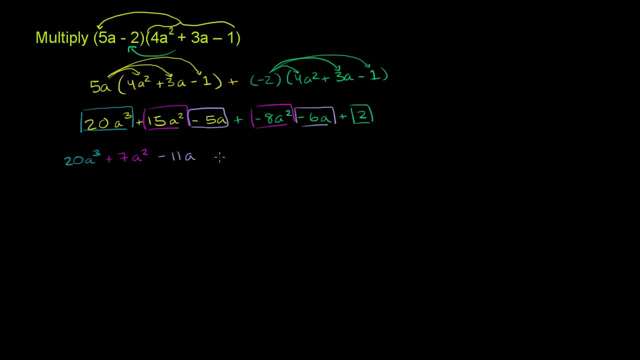 And then, finally, we have this constant out here, this plus 2.. Now I'll show you another way to get this exact same answer. And we are done. We have simplified, We've combined all our like terms. Another way to do this, which is essentially: 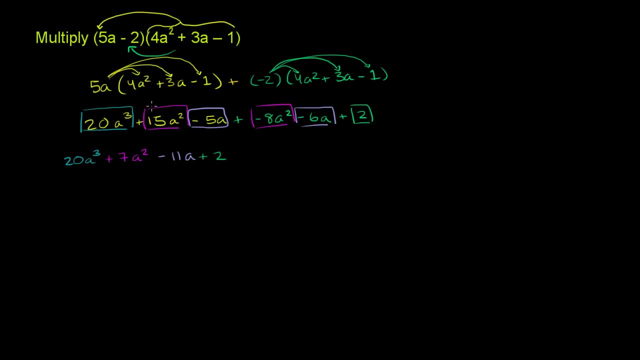 just doing the distributive property twice, but it's essentially more analogous to how we actually multiply numbers. So if we do it like this, we can actually take this expression up here: 4a squared plus 3a minus 1, and then multiply it by this second expression. 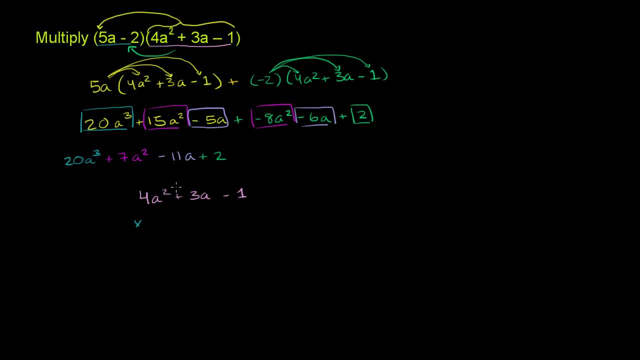 right over here. So times and I'll write it in the same places. And when I talk about places here, I'm not talking about powers of 10. I'm talking about powers of a. So this is, in the first, power of a space. 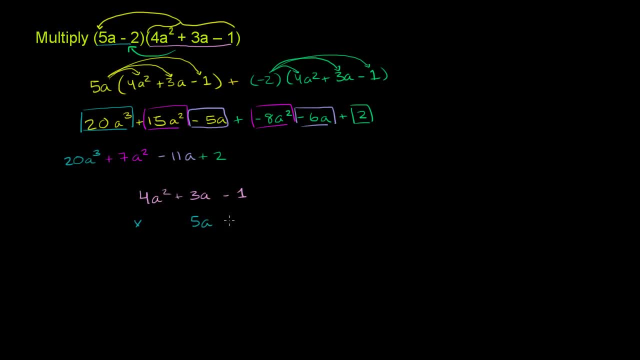 So 5a. see we have first powers of a in this space minus 2.. This is 0th power of a. This is the a to the 0th power space instead of the ones place. This is the a to the first power instead of the tens place. 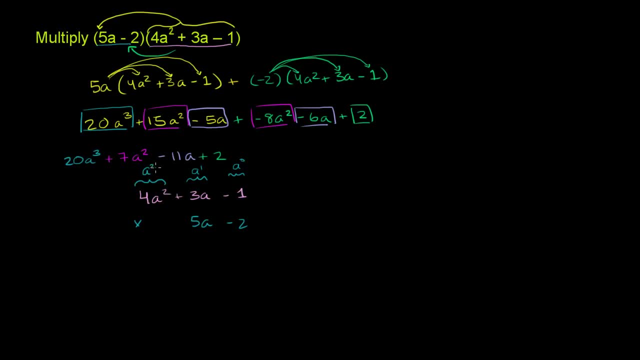 And this is a to the squared power place instead of the hundreds place. But it's completely analogous to what you do when you learn to multiply numbers in the first or second grade. So let's multiply these. So first, let's multiply negative 2. 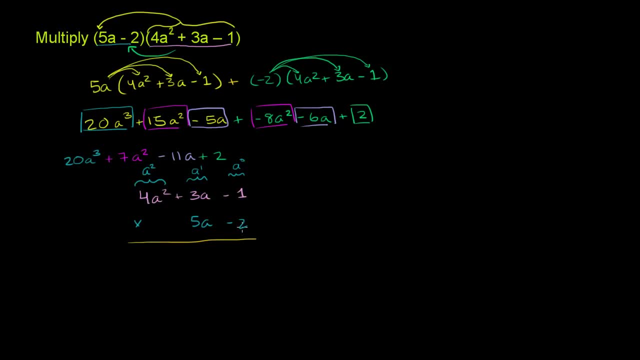 times this entire thing. Remember, we're just essentially doing the distributive property When I multiply negative 2 times this entire thing. I'm doing this step right over here. So negative 2 times negative 1 is positive 2. And once again, there's no a there. 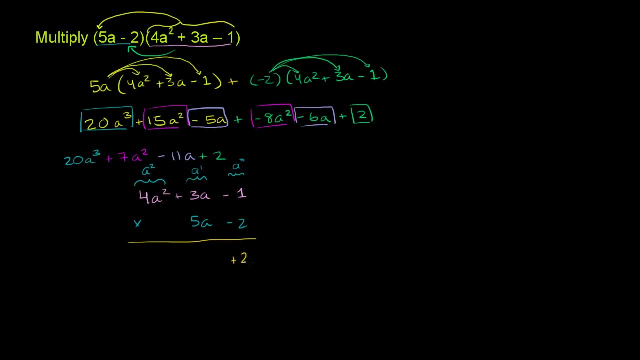 so I'm going to write it in the a to the 0 space or the ones place. So it's going to be positive 2.. Negative 2 times 3a: well, that is negative 6a And it's going to be in the a place. 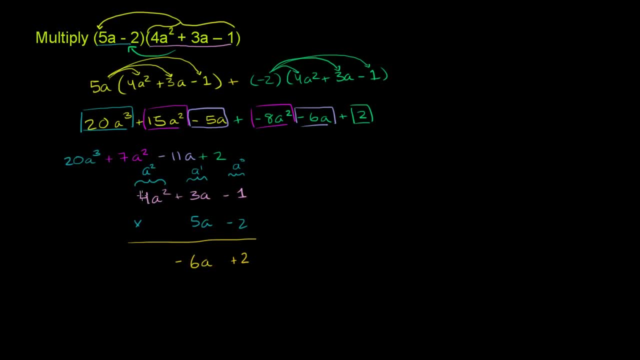 Negative 6a a to the first power place, And then negative 2 times 4a squared. well, that's just going to be negative 8a squared. So this is negative 2. being multiplied by all of that, It gives me this: 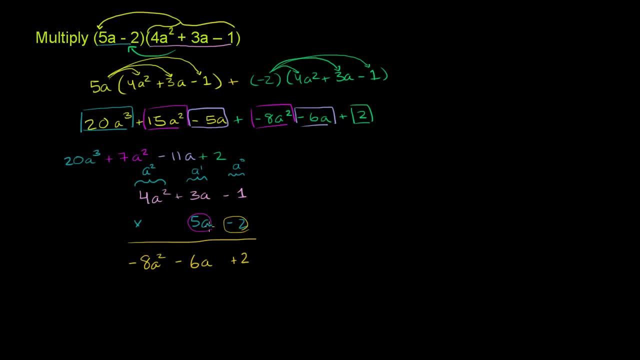 And then when I take my 5a and I multiply it by negative 1, that's negative 5a And so it goes into the a place. so negative 5a, It goes under a like term. Then 5a times 3a. 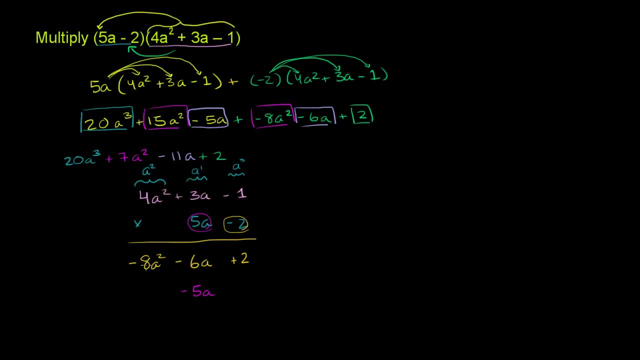 5 times 3 is 15.. a times a is a squared, So it goes under the other a squared, So it's 15a squared. And then finally, 5a times 4a squared. 5 times 4 is 20.. 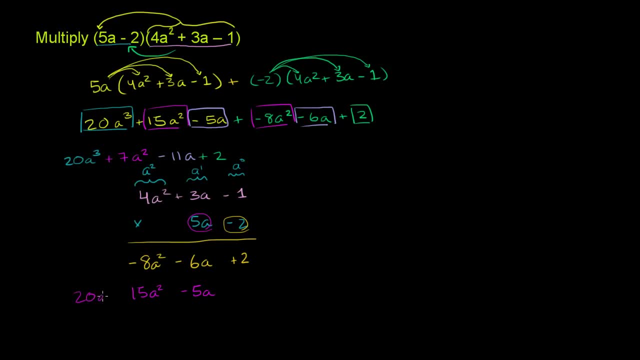 a times a squared is a to the third, So you have 20a to the third, And now you can just add it all up And we get 2 plus nothing is 2.. Negative 6a minus 5a- well, that's just negative 11a. 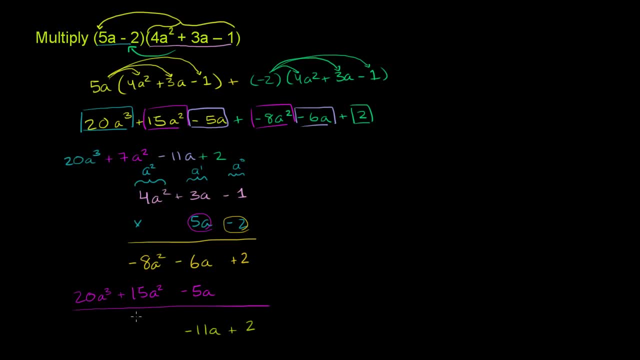 We still have this plus 2 here, Negative 8a squared plus 15a squared. Well, that's going to be 7a squared, So plus 7a squared, And then you're adding this to nothing, So you have 20a to the third. 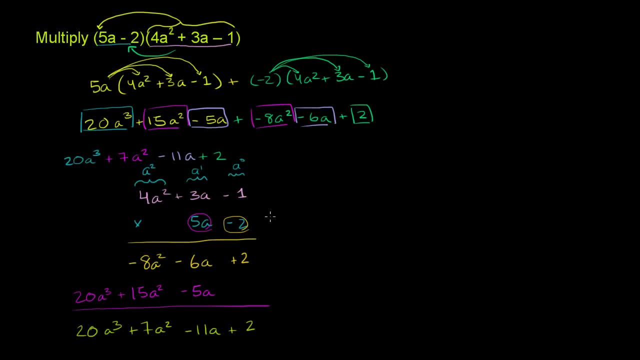 And we got the exact same answer, Because we really just did the same exact thing, We just wrote it in a different way.